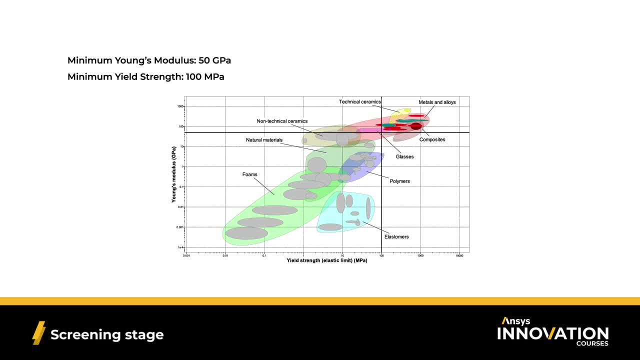 Now I place my line for yield strength at 100 megapascals. For values greater, I'm considering every material to the right of this line. So if we zoom in and remove all unsuitable materials, we end up with 22 candidates. 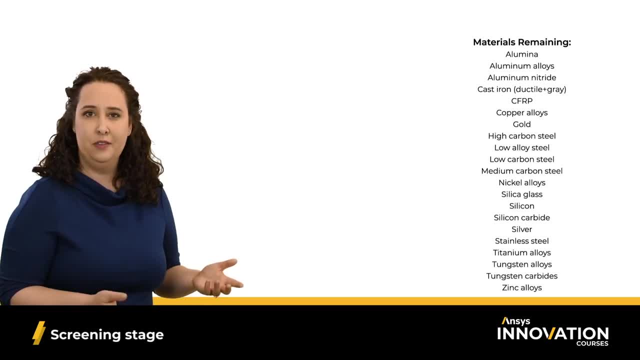 which are shown here. Well, are all of these materials suitable candidates? It can be tough when looking at so many options- And yes, 22 is a lot- when you're trying to pick the optimal material for the job. Looking at this list, I can already see a material that's not going to work. 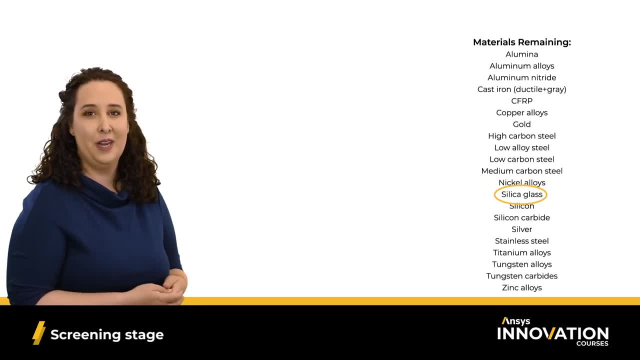 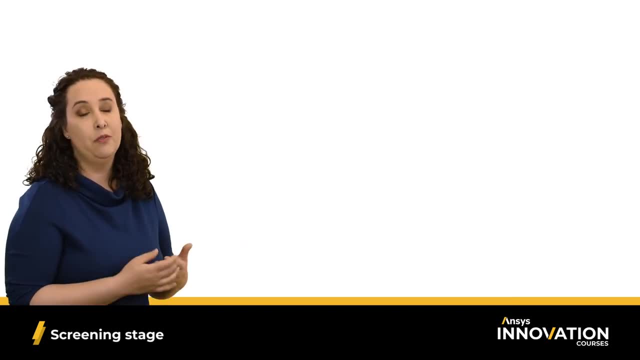 Silica glass Glass is not a suitable material for an airplane wing, So that means we need to go back to our design criteria and continue screening to remove all unsuitable materials. So next on our list was toughness or the fracture toughness of our material. 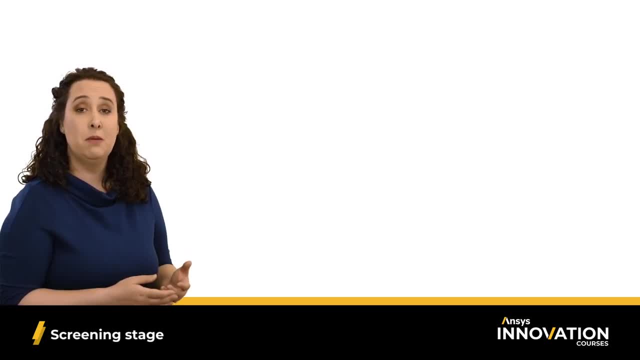 Again, based on some background research, we know that the material is not suitable for an airplane wing. We need a minimum value of 15 megapascals per meter to the one half for the fracture toughness of our material for this airplane wing. 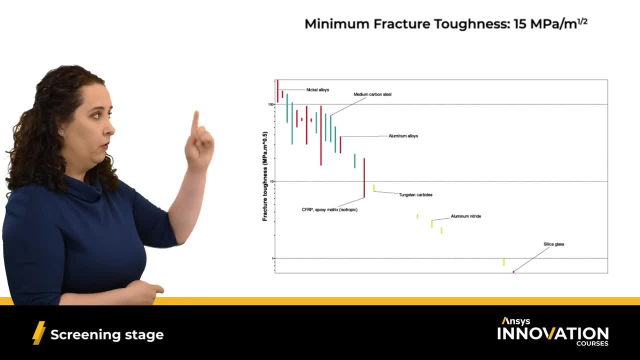 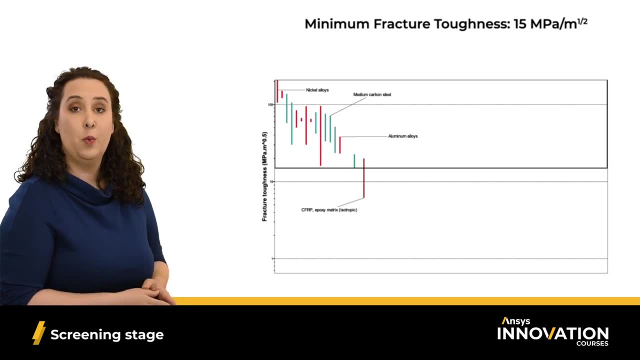 So let's plot fracture toughness in a bar chart where fracture toughness is along the y-axis. If I draw a line at 15 megapascals per meter to the one half and I only consider materials above that line, we can see that silica, glass and all of our technical ceramics such as tungsten carbide. 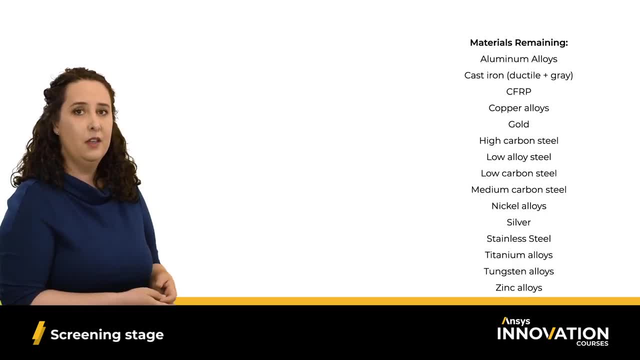 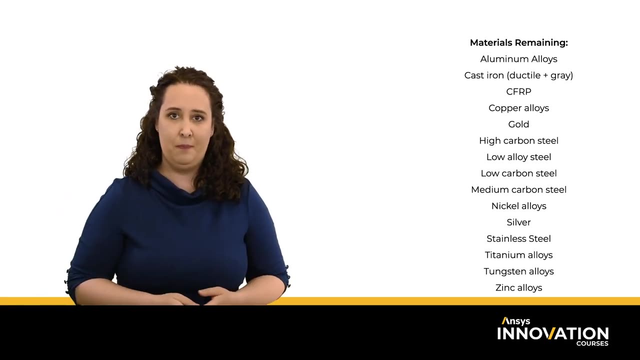 are removed from consideration. Looking at this list, we now see that we only have metals and one composite made of carbon fiber left. Now, metals and composites seem quite reasonable for materials to make an airplane out of. so we're actually done with the screening process, But I still have 16 material candidates left. 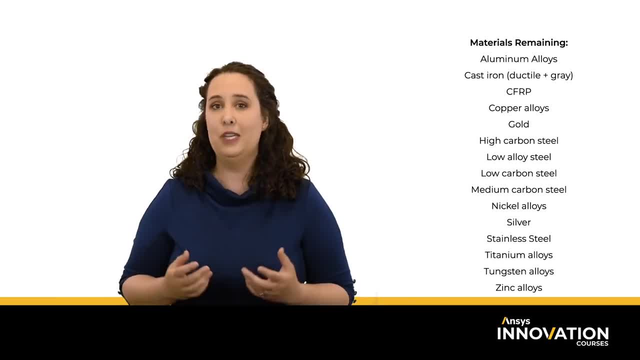 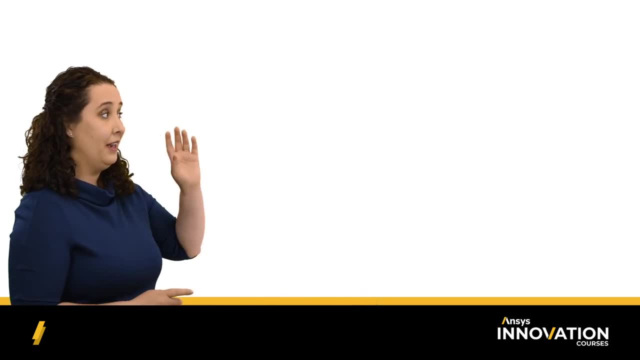 Now I can move on to ranking, where I'm trying to optimize my choice based on the materials I have left. So let's go back to our design criteria and see if we have any material left. So, once again, going back to our design criteria, we see that 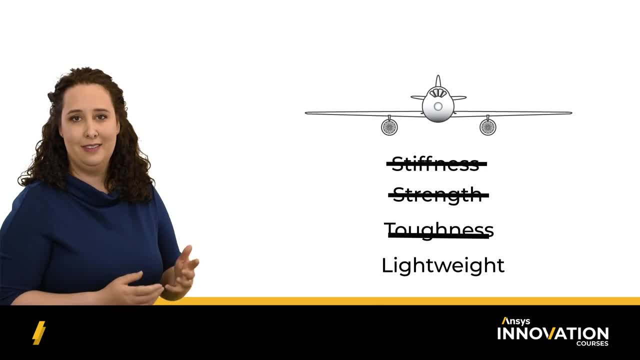 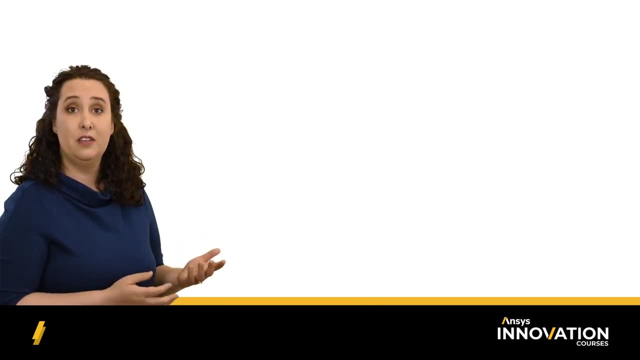 the material needs to be lightweight. That's our last criteria that we need to consider. So in this case, we're going to use density to help us do this. So let's plot density as a bar chart, once again putting density on the y-axis. 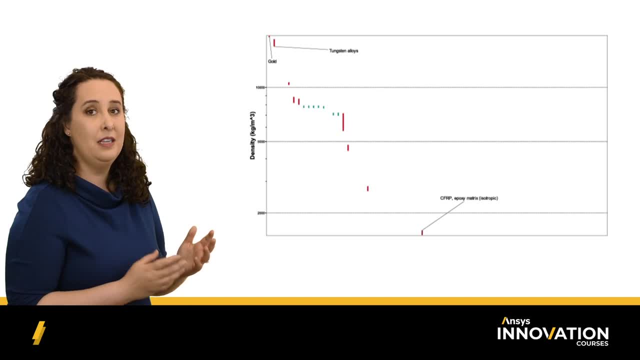 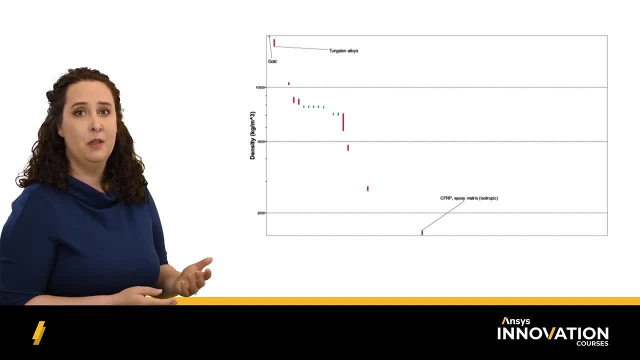 But what about materials like steel or aluminum? All of our ferrous alloys are shown on this chart in teal over here, And aluminum is a very lightweight metals we can see here, but it's not quite as light as our carbon fiber composites. 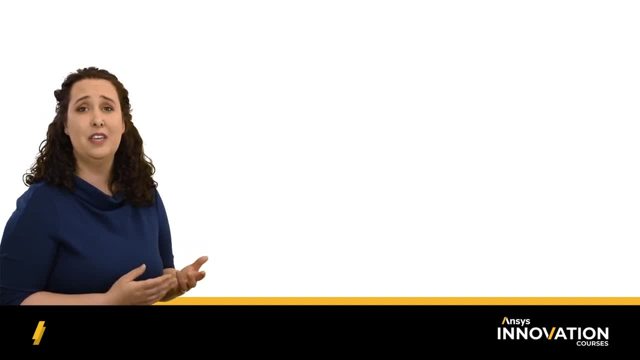 This ranking doesn't seem very clear. There's something else we could consider. I could consider price. if I am part of a company that manufactures airplanes, I need to be considering price when I'm choosing a material to build these planes out of. So let's add price to the x-axis and compare density to price for our ranking. 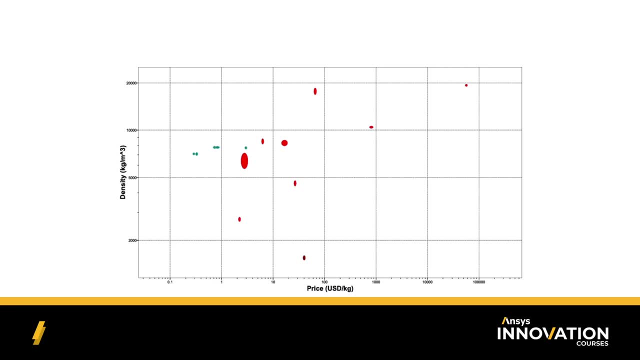 Now we start to see something interesting. I want the cheapest and lightest materials, which are located in the bottom left-hand corner of my chart. down here We can see three materials really stand out from the rest of the group. The cheapest but heaviest materials are: 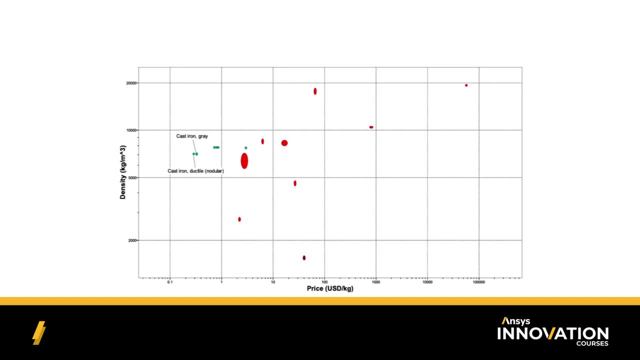 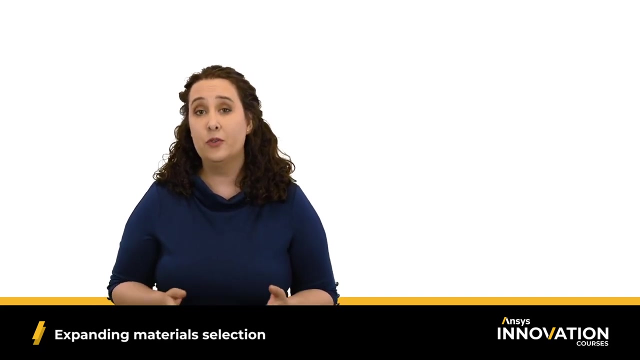 cast irons, both ductile and gray. The lightest but most expensive is our carbon fiber composite, And somewhere in the middle are aluminum alloys, which are often used in the aerospace industry. Now, this is just a simple example. There are hundreds of grades of aluminum that 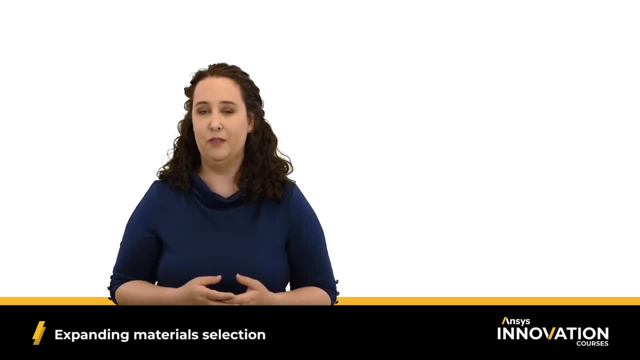 we would need to consider in order to select our final material for our airplane wing, but we've shown that we're able to use our Ashby charts to quickly and effectively narrow down our material. So let's take a look at some of the materials that we need to consider in order to 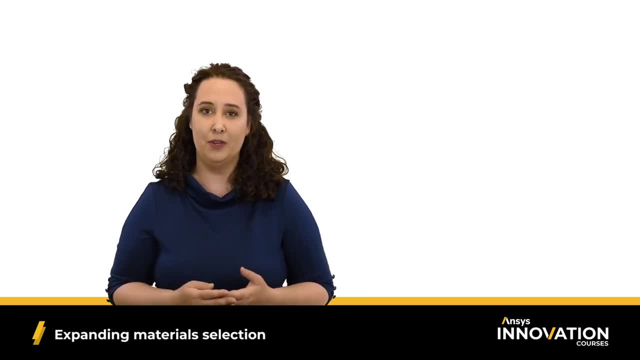 select our final material for our airplane wing. But we've shown that we're able to use our Ashby charts to quickly and effectively narrow down our material choices, much faster than using tables of numbers. Now you might be thinking to yourself: can I take this further? Can I use this to? 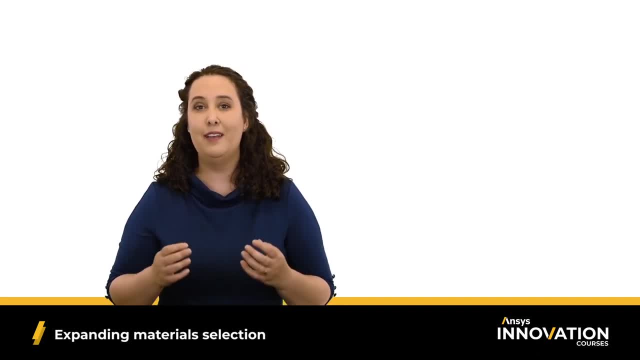 logically select materials for advanced applications? And the answer is yes. The Ashby selection methodology- yes, the same Ashby as our Ashby charts- is a logical workflow that allows people to work on complex material selection problems. In fact, Granta EduPack and Granta Selector.